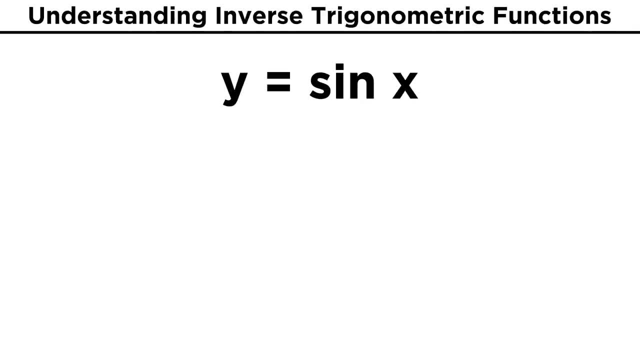 function. Now let's try: y equals sine x. If we swap the variables, how do we solve for y? The only way to do this is through a square to take the inverse sine of both sides. This will cancel out the sine operating on Y and we get Y equals inverse sine X. 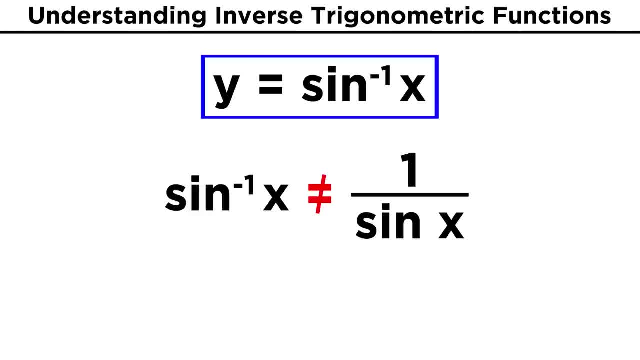 We must note that inverse sine X is not the same thing as one over sine X. If we had the quantity sine X to the negative one power, that would equal one over sine X, which we already know is cosecant X. Instead, when we have the negative one here, it's the inverse sine function, and rather 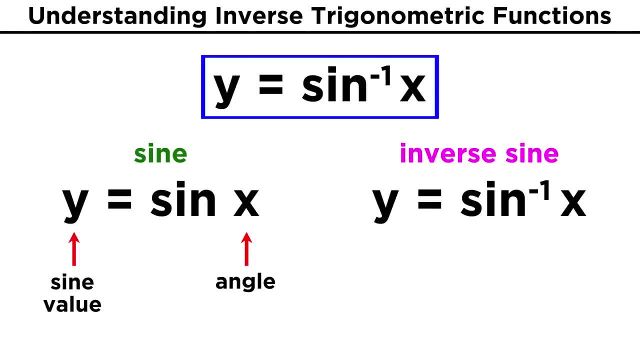 than sine X, where you plug in an angle and get a sine value. for inverse sine X. you plug in a valid sine value and it gives you the angle that generates it. Inverse sine can also be represented this way as arcsine X. 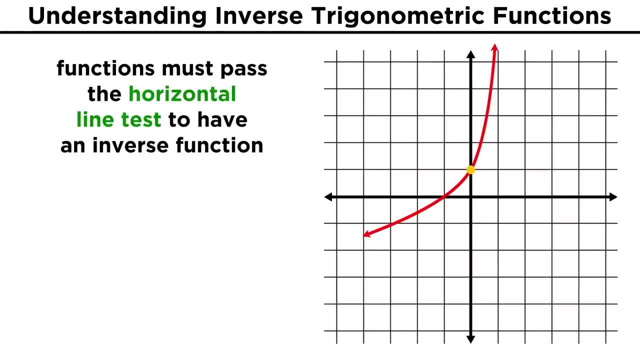 Inverse sine can also be represented this way as arcsine X. We should quickly note that in order for a function to have an inverse function, it must pass the horizontal line test, because when we find the inverse, we are reflecting the function across the line Y equals X and whatever we get must pass the vertical line. 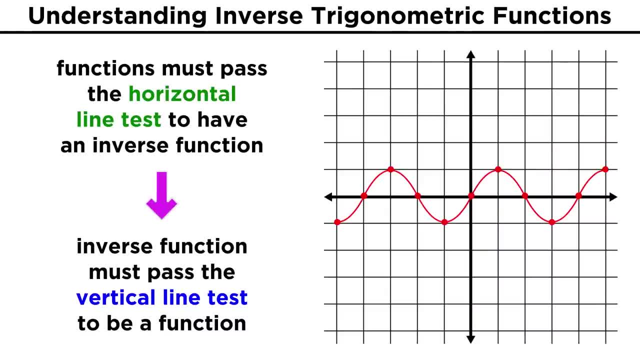 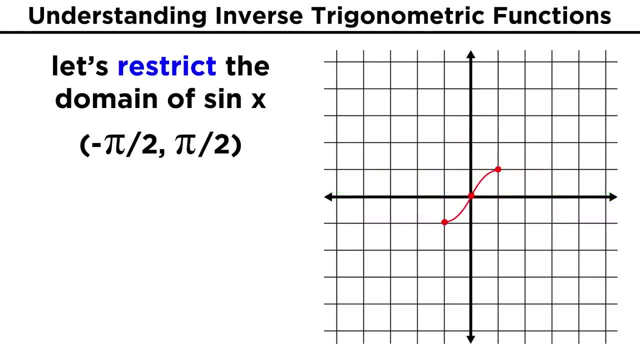 test to be considered a function. So sine X as a whole does not have an inverse function, but we will instead look at a restricted domain. This section does pass the horizontal line test and it is the inverse of this section that gives us the inverse sine function, which will look like this: 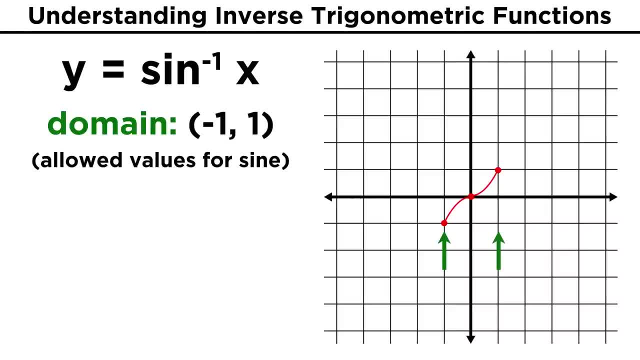 The domain of this function will be negative one to one, because those are the only sine values that are possible. The range will be negative- half pi to half pi- because those are the angles we get when we plug in each possible unique sine value. 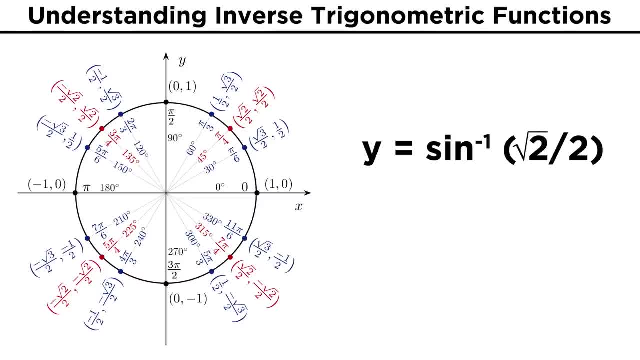 So let's make sure we know how to evaluate these. What is the inverse sine of root? two over two? Well, if we recall our unit circle, the angle that gives a sine of root two over two is quarter pi. so the inverse sine of root two over two is quarter pi. 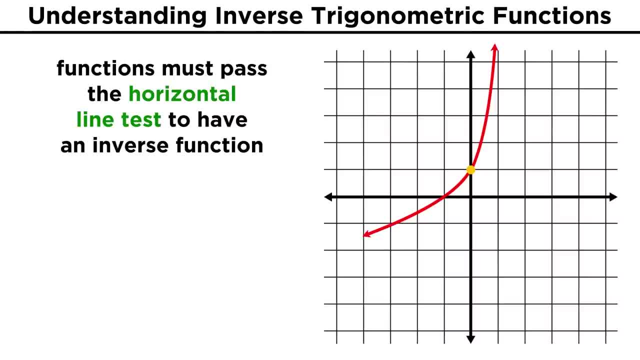 We should quickly note that in order for a function to have an inverse sine function, it must pass the horizontal line test, because when we find the inverse, we are reflecting the function across the line Y equals X and whatever we get must pass the vertical line. 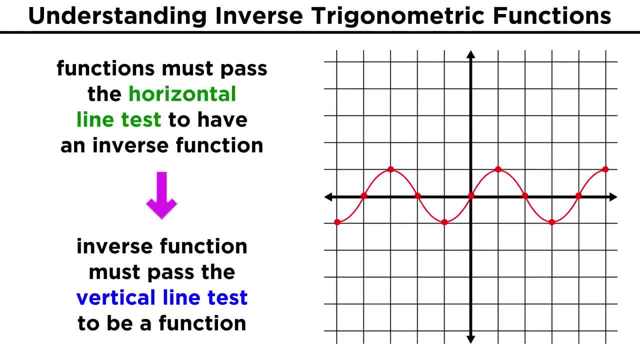 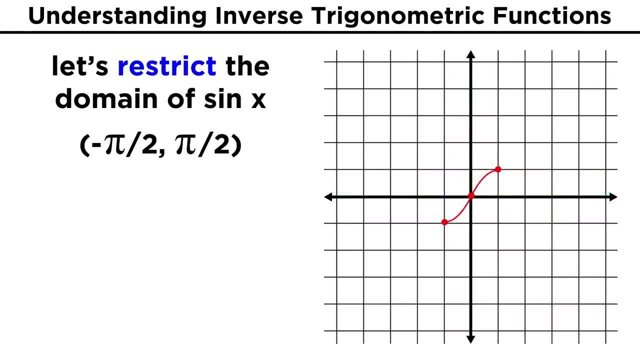 test to be considered a function. So sine X as a whole does not have an inverse function. but we will instead look at a restricted domain for this function from negative half pi to half pi. How do we do this? Let's see. 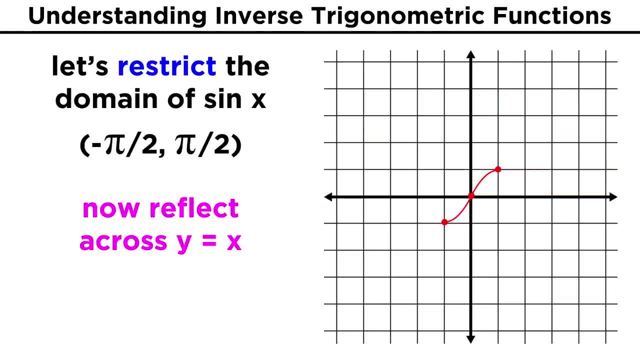 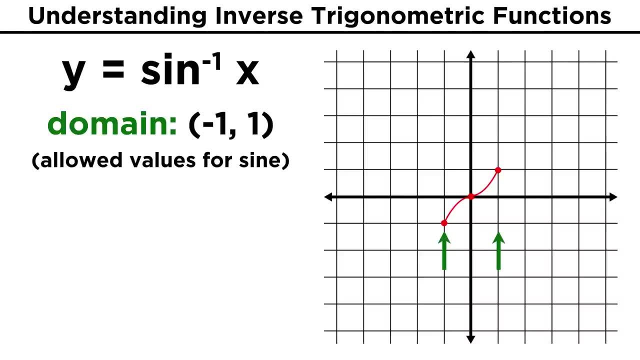 does pass the horizontal line test, and it is the inverse of this section that gives us the inverse sine function, which will look like this: The domain of this function will be negative one to one, because those are the only sine values that are possible. 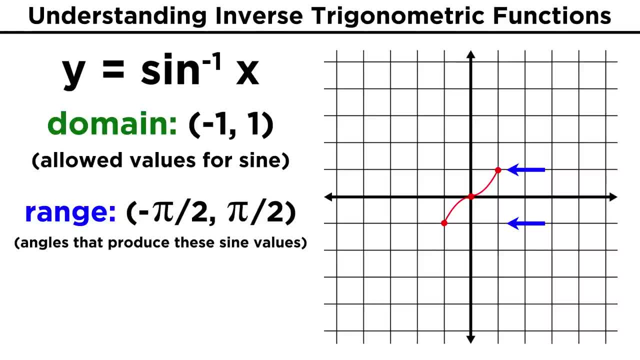 The range will be negative- half pi to half pi- because those are the angles we get when we plug in each possible unique sine value. So let's make sure we know how to evaluate these. What is the inverse sine of root? two over two. 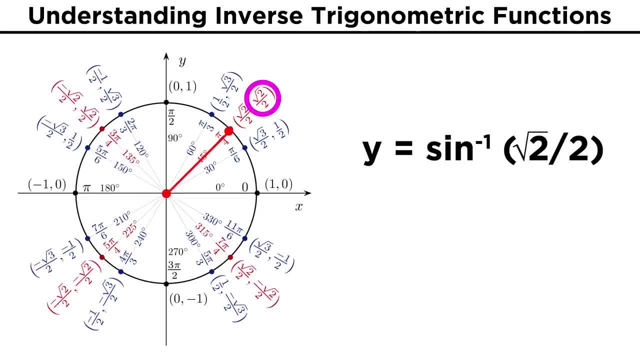 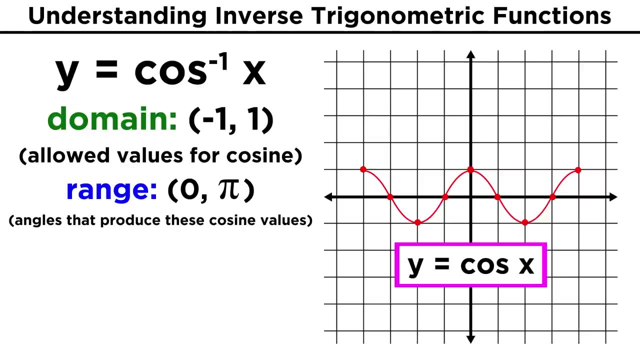 Well, if we recall our unit circle, the angle that gives a sine of root two over two is quarter pi. so the inverse sine of root two over two is quarter pi. Now let's move on to inverse cosine. This will be the inverse of cosine X, from zero to pi. 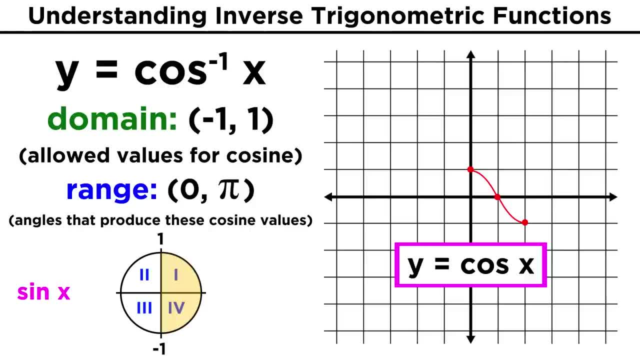 This is a different restriction than we had for sine, because sine goes to the sine, of negative one to positive one, as it moves through quadrants. four and one Cosine spans all the possible values, from one to negative one, as it goes through quadrants. 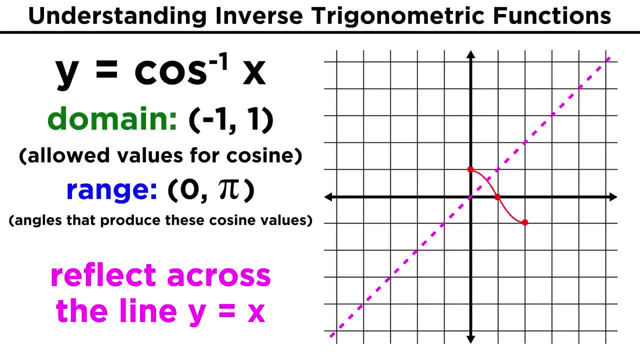 one and two. so we take the graph of cosine X from zero to pi and we reflect it across the line Y equals X to get the inverse cosine function. As we would expect, the domain is negative one to one and the range is zero to pi. 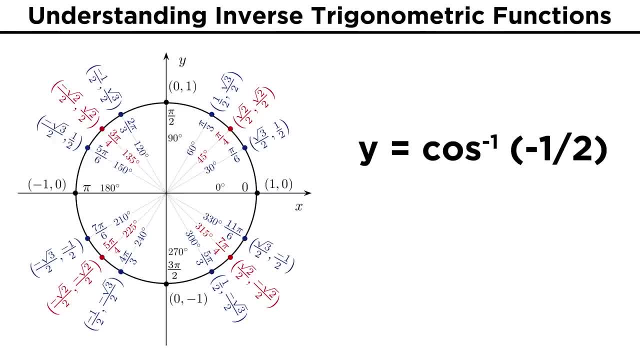 What is the inverse cosine of negative one half? Well, that would be the angle in this interval that gives a cosine value of negative one half, and if we remember the unit circle, we know that must be two thirds pi. Now let's look at inverse tangent. 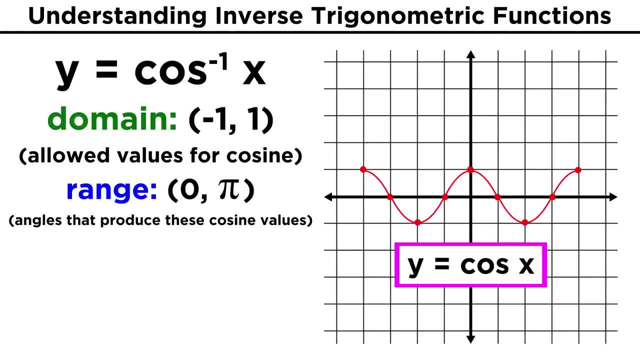 Now let's move on to inverse cosine. this will be the inverse of cosine X from zero to pi. This is a different restriction than we had for sine, because sine goes from negative one to positive one as it moves through quadrants four and one. 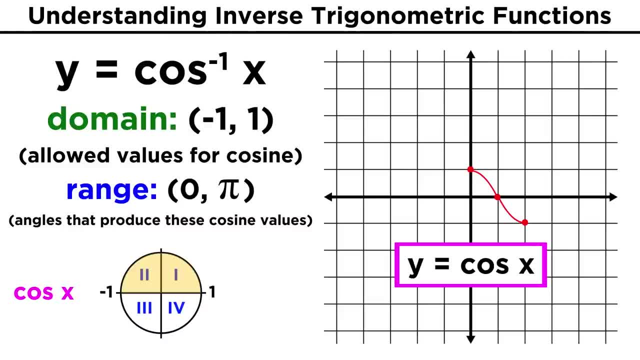 Cosine spans all the possible values, from one to negative one, as it goes through quadrants one and two. so we take the graph of cosine X from zero to pi and we reflect it across the line Y equals X to get the inverse cosine function. 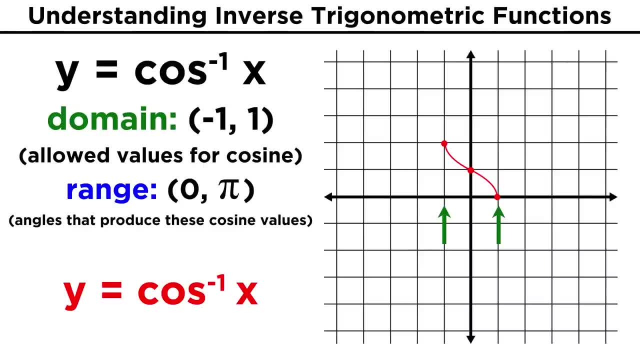 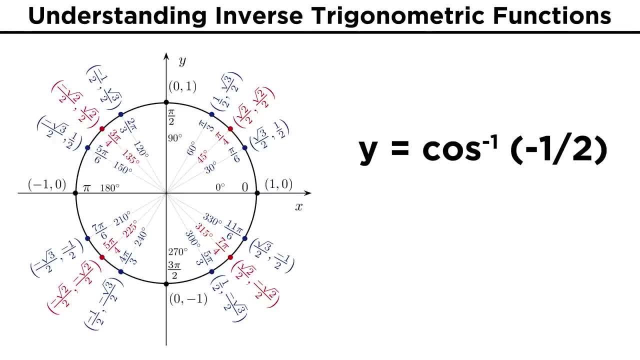 As we would expect, the inverse sine of root two over two is the inverse sine of root two. in fact, the domain is negative one to one and the range is zero to pi. What is the inverse cosine of negative one half? Well, that would be the angle in this interval that gives a cosine value of negative one. 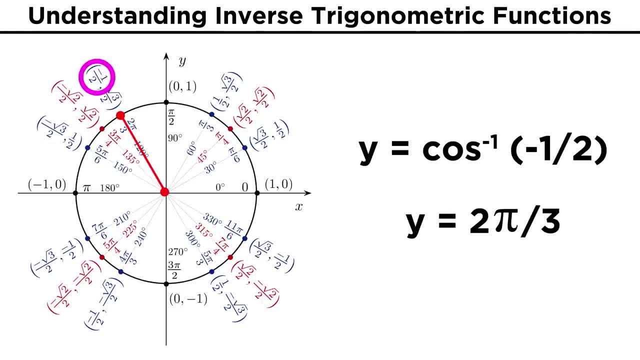 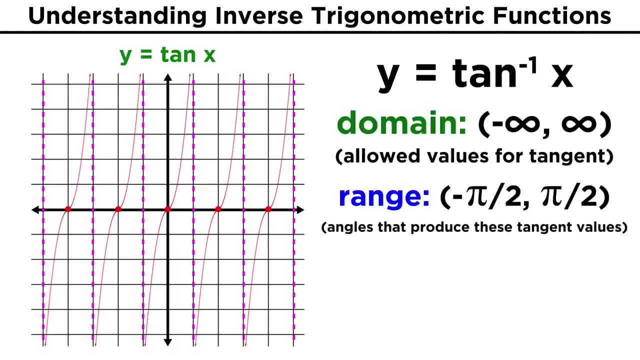 half, and if we remember the unit circle, we know that must be two thirds pi. Now let's look at inverse tangent. Starting with tangent X, we see that we will want to restrict things, so we're going to plug in all the possible tangent values to within negative half pi and half pi. so 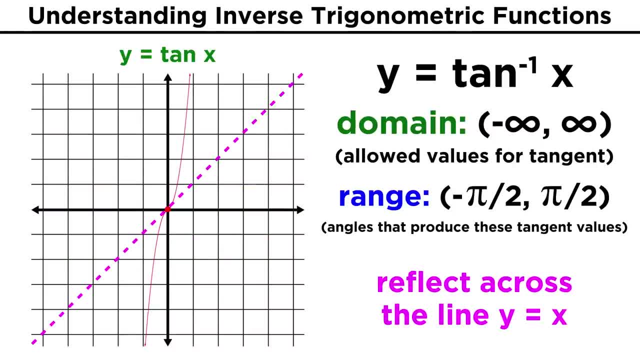 that it passes the horizontal line test. Now to get the inverse tangent function, we reflect across: Y equals X and we get this. Now the domain is all real numbers, while the range is negative- half pi to half pi, since those are the angles we get when we plug in all the possible tangent values, which 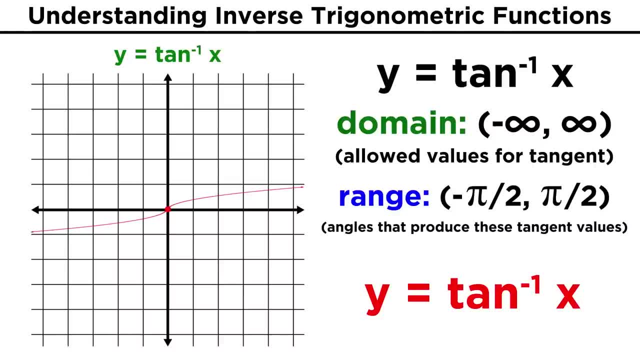 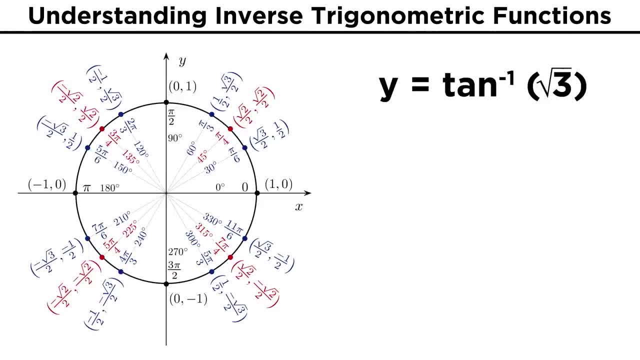 go towards positive and negative infinity as cosine gets very small. These are trickier to evaluate in your head but sometimes we can do it. like the inverse tangent of root three, We might realize that the angle that produces a tangent of root three must have a sine value. 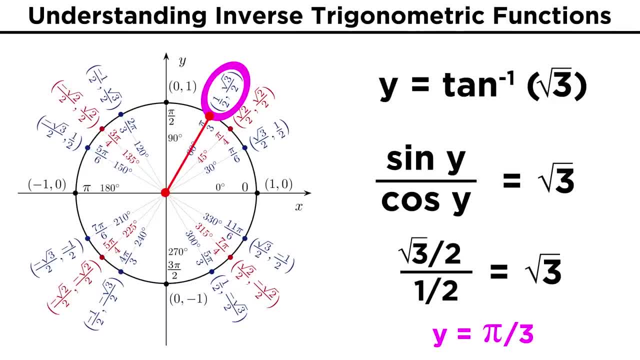 over a cosine value that equals root three, and of the common angles, that must be a third pi, since root three over two, divided by one half, is the same as root three over two times two, which equals root three. Luckily, rather than having to evaluate inverse trig functions by hand, we can always just 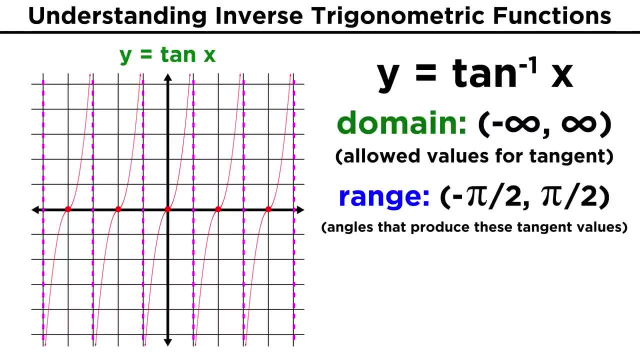 Starting with tangent X, we see that we will want to restrict things to within negative half pi and half pi, So that it passes the horizontal line test. Now to get the inverse tangent function, we reflect across: Y equals X and we get this. 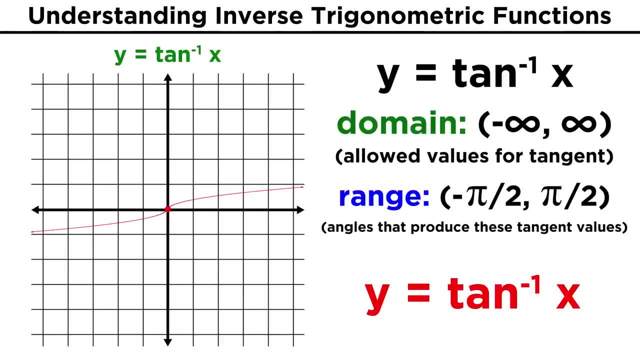 Now the domain is all real numbers, while the range is negative: half pi to half pi, since those are the angles we get when we plug in all the possible tangent values which go towards positive and negative infinity. as cosine gets very small, These are trickier to evaluate in your head, but sometimes we can do it. 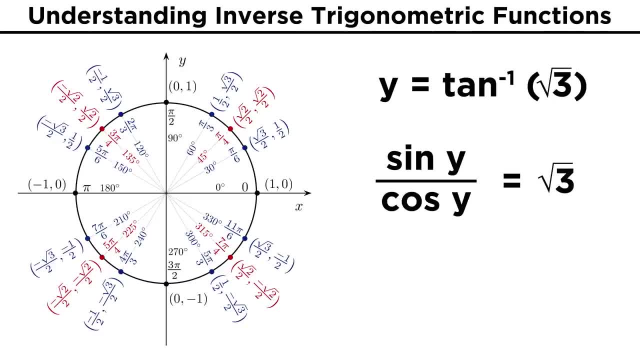 Like the inverse tangent of root three. We might realize that the angle that produces a tangent of root three must have a sine value over a cosine value that equals root three, and of the common angles, that must be a third pi, since root three over two, divided by one half, is the same as root three over two times. 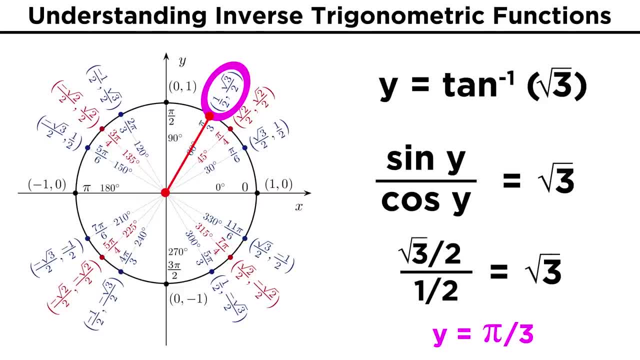 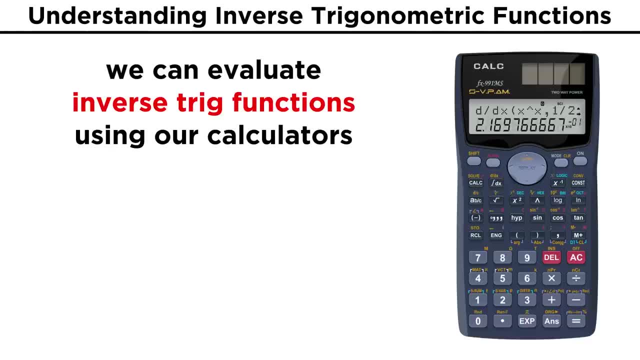 two, which equals root three. Luckily, rather than having to evaluate inverse trig functions by hand, we can always just plug them into a calculator. Just make sure it's in radian mode, plug in the sine cosine or tangent value and 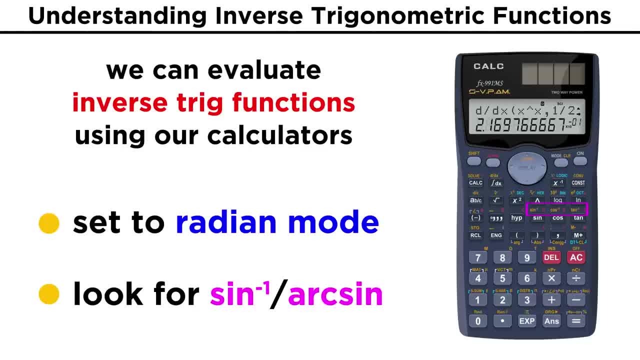 use the buttons that say things like inverse, sine or arcsine to find out what the corresponding angle is. Just remember: you may get a messy answer that will be hard to express as fractions of pi, but it will be the correct answer. Let's check comprehension. 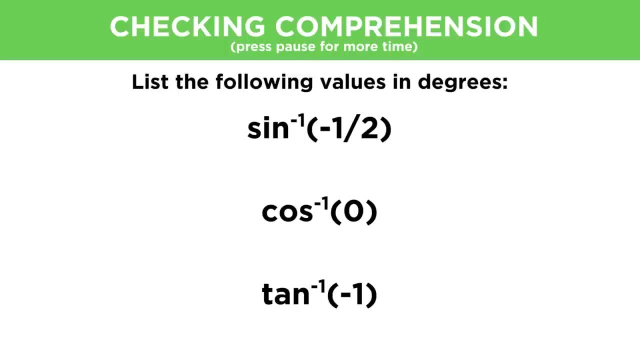 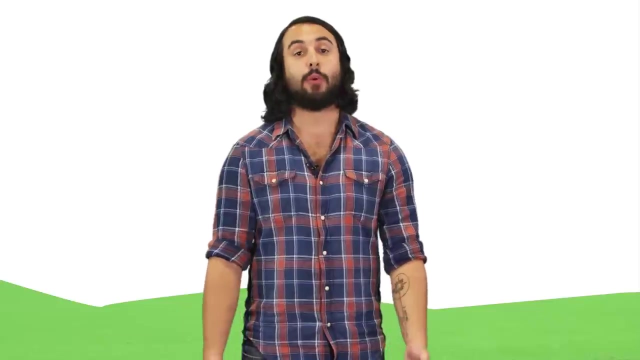 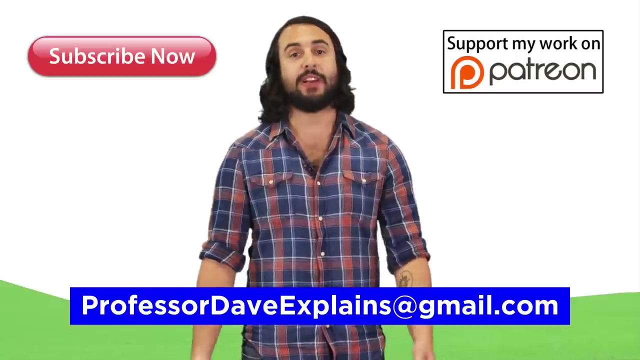